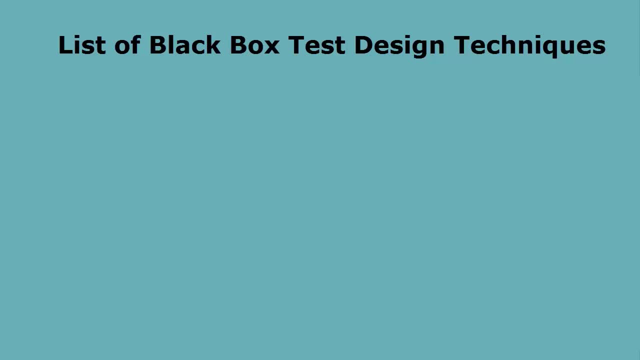 techniques. First one: equivalence, partitioning, boundary value analysis, decision table, state transition, exploratory testing and, last, error, guessing. In this video we see what are these techniques and why we use. In the upcoming videos we see each technique in detail with practical examples. 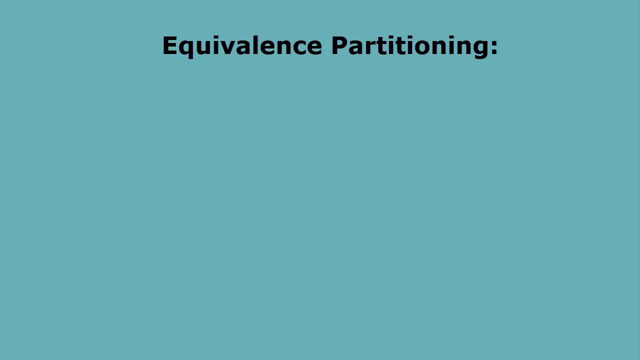 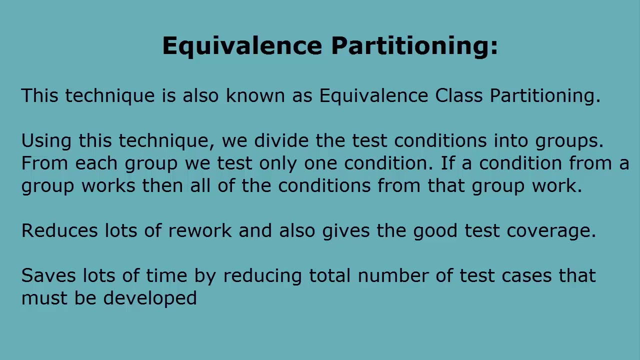 First technique in our list is equivalence partitioning. This technique is also known as equivalence class partitioning. Using equivalence partitioning test design techniques, we divide the test conditions into partitions. For each partition we do test only one condition. Assumption is that all the conditions in one 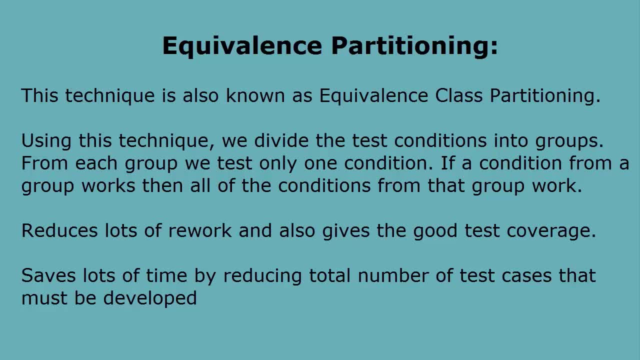 partition works in the same manner. If a condition from a partition works, then all the conditions from that partition will work. This technique reduces lots of rework and also gives good test coverage. We could save lots of time by reducing total number of test cases that. 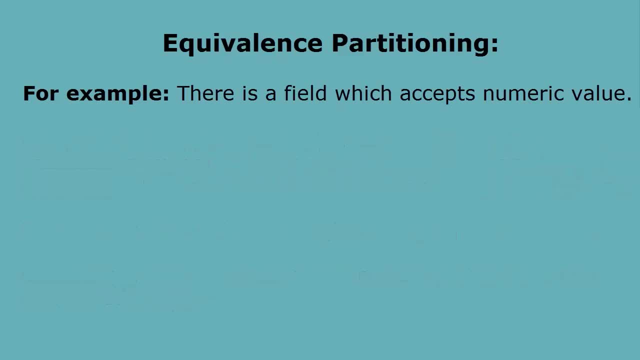 must be developed. For example, there is a field which accepts numeric value. In this case, we split the test conditions as enter numeric value, enter alpha numeric value, enter alphabets, and so on. We need to test only one condition from each partition. This is because we are assuming. 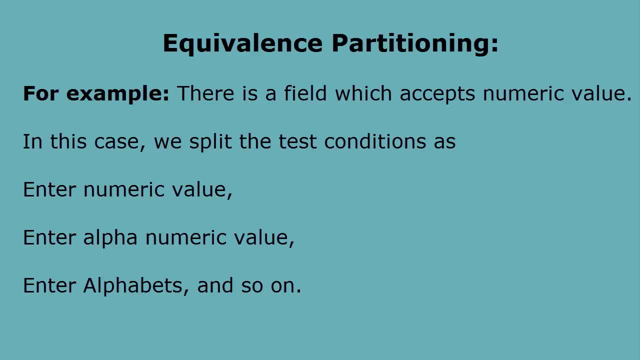 that all the conditions in one partition works in the same manner. If one condition in a partition works, then all the conditions in that partition will work. As I mentioned earlier, we will see in detail and practical examples on this in the next video. 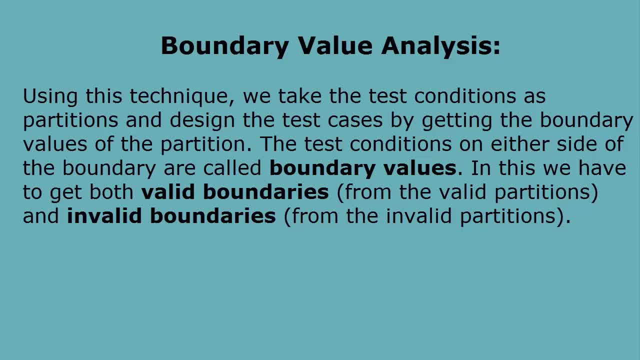 Boundary value analysis. Using this technique, we take the test conditions as partitions and design the test cases by getting the boundary values of the partition. The boundary between two partitions is equal to the place where the behavior of the application varies. The test conditions on either side. 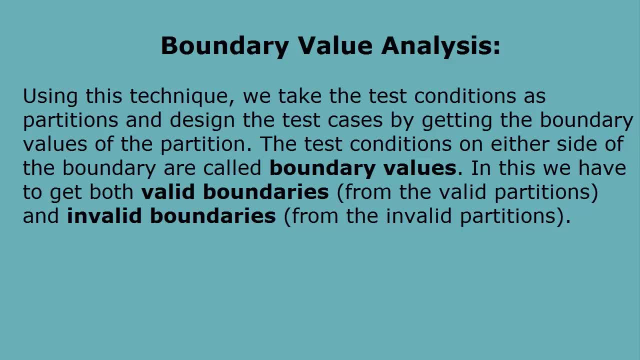 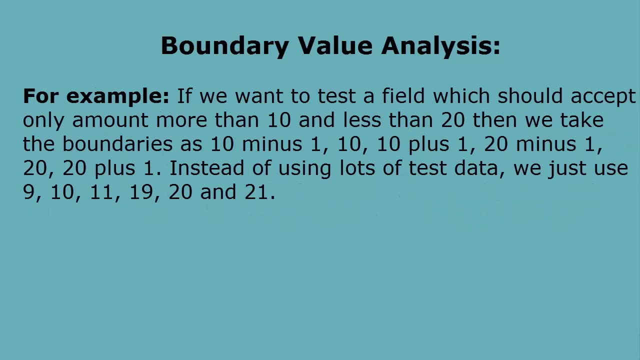 of the boundary are called boundary values. In this we have to get both valid boundaries and invalid boundaries. For example, if we want to test a field which should accept only amount more than 10, then we have to get the test condition as part of the test field. 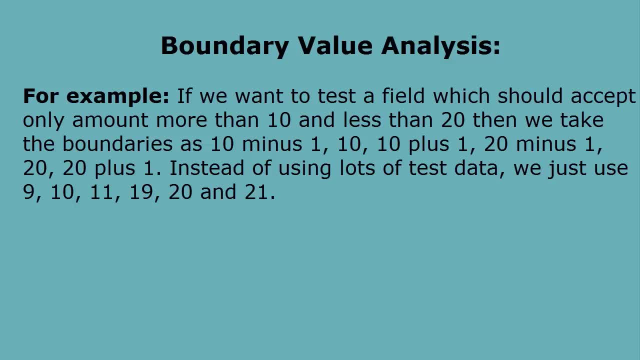 Then we take the boundaries as 10-1, 10, 10 plus 1,, 20-1, 20,, 20 plus 1.. Instead of using lots of test data, we just use 9,, 10,, 11,, 19,, 20 and 21.. 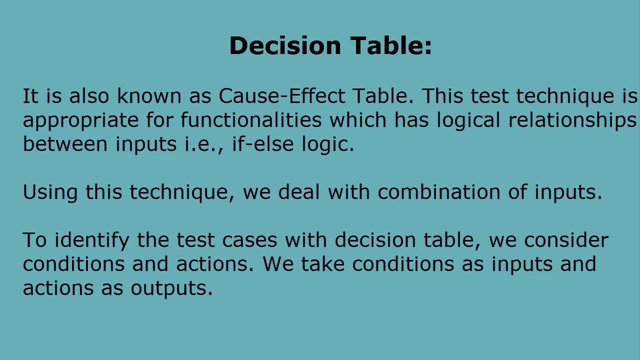 3. Decision Table. It is also known as cause-effect table. This test technique is appropriate for functionalities which has logical relationship between inputs, ie if-else logic. In decision table technique we deal with combination of inputs To identify the test. 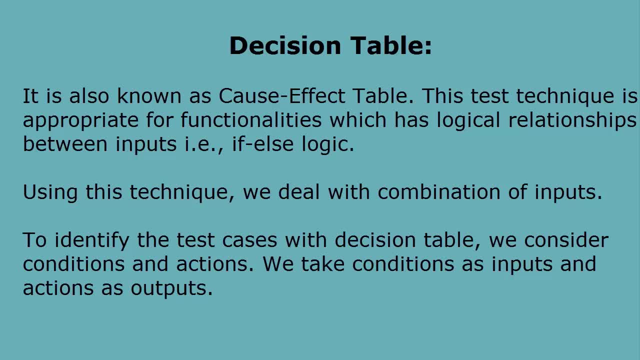 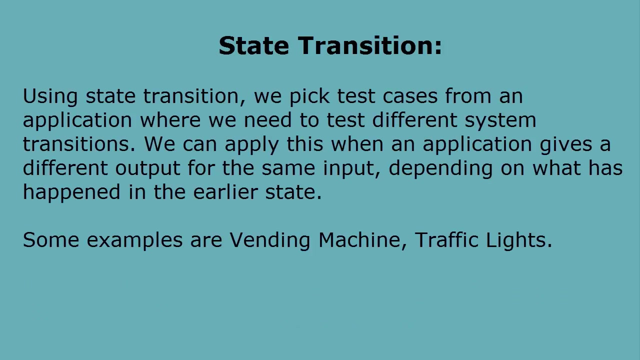 cases with decision table. we consider conditions and actions. We take conditions as inputs and actions as outputs. We'll explain what are conditions and actions in detail in next video. 3. State Transition: We pick test cases from an application where we need to test different system transitions. 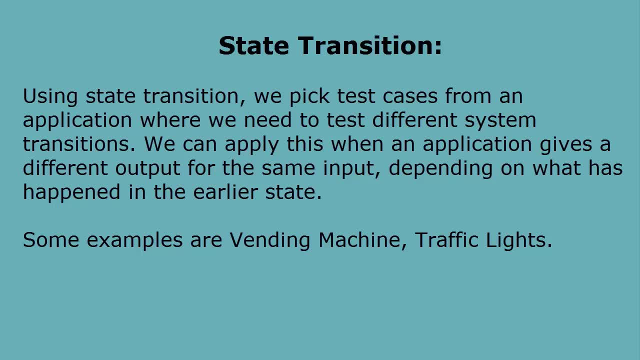 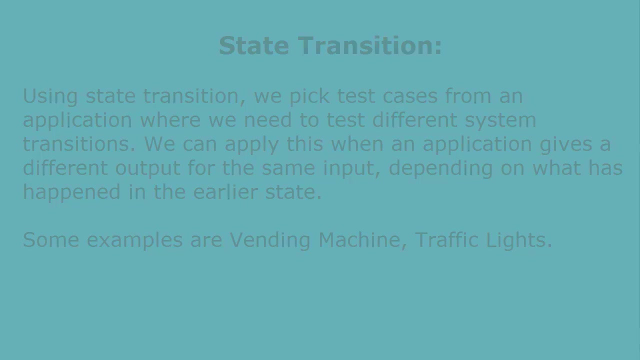 We can apply this when an application gives a different output from the same input, depending on what has happened in the earlier state. Some examples are vending machine traffic lights. Vending machine dispenses products when the proper combination of coins is deposited. Traffic lights will change sequence when cars are moving or waiting. 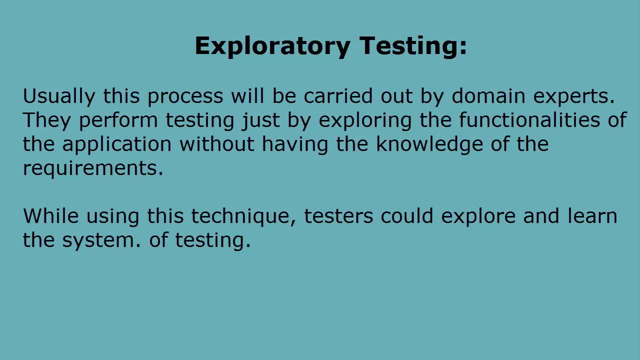 Severeity testing. Usually, this process will be carried out by domain experts. They perform testing just by exploring the functionalities of the application, without having the knowledge of the requirements. While using this technique, testers could explore and learn the system. High severity bugs are found very quickly in this type of testing.